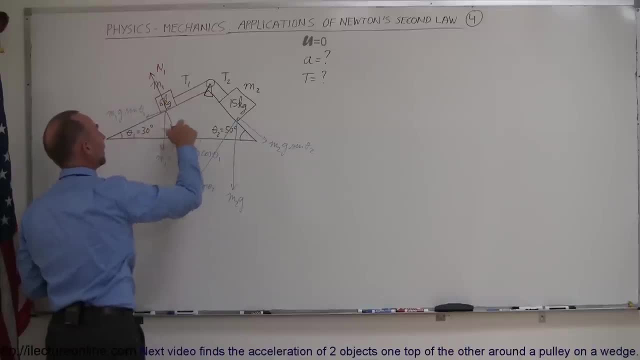 opposite in direction to m1 g cosine theta, 1 equal in magnitude. And then, of course, here we have n2.. Again, it's equal in magnitude to m2 g cosine theta, and opposite in direction, So that these cancel each other out. These cancel each other out. Of course, this one is gone, because I divided that into the components. That one is gone as well. So we only have two forces left, which is this force, m1 g sine theta, pulling the whole system in this direction, And 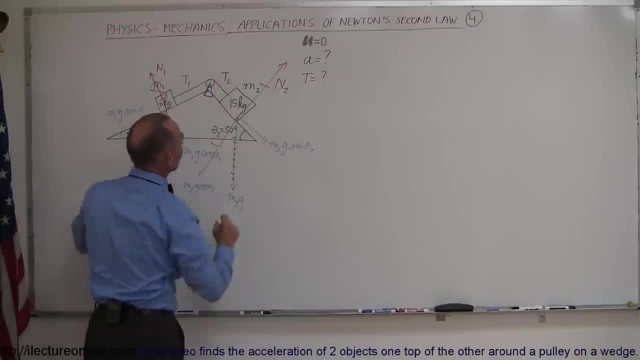 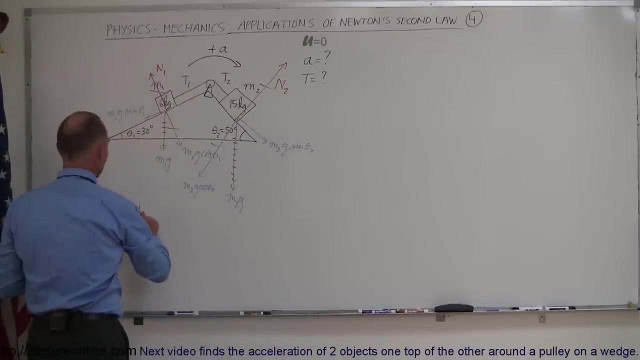 here we have m2 g sine theta 2, pulling the whole system in this direction, This being a heavier object on a steeper incline. I would think that this is a bigger force than this and therefore I would assume that the whole system would be accelerating in this direction. So I'm going to call acceleration in this direction to be the positive direction. Now I'm using Newton's second law that says f net is equal to mass total times acceleration. If I then 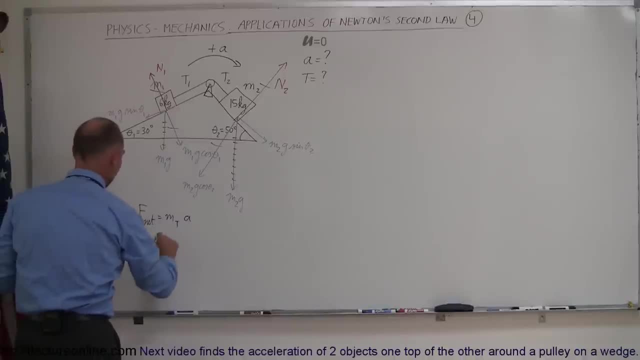 rearrange that equation to solve for a. a is equal to f net divided by m total. And of course the net force would be all the forces aiding the acceleration minus all the forces opposing the acceleration. This one is aiding, this one is opposing. So this would become m2 g sine of theta 2 minus m1 g sine of theta 1.. That would be the net force acting on the system divided by m2 g sine of theta 2.. 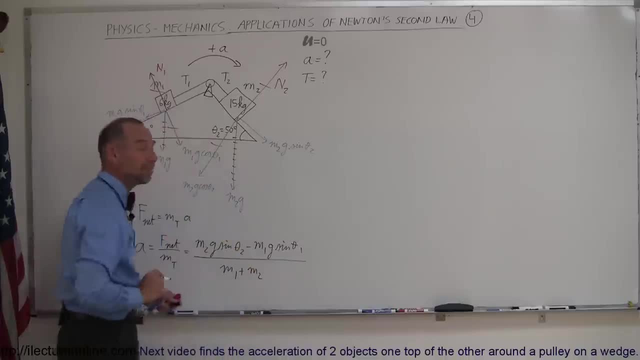 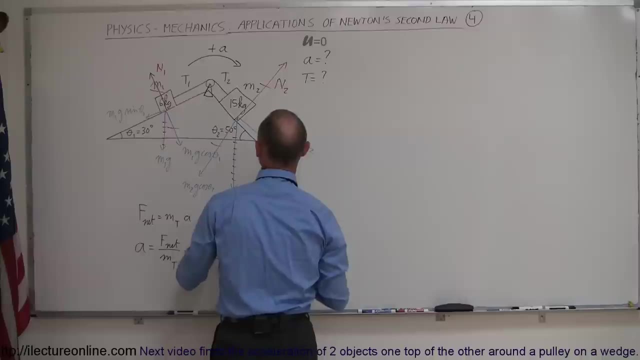 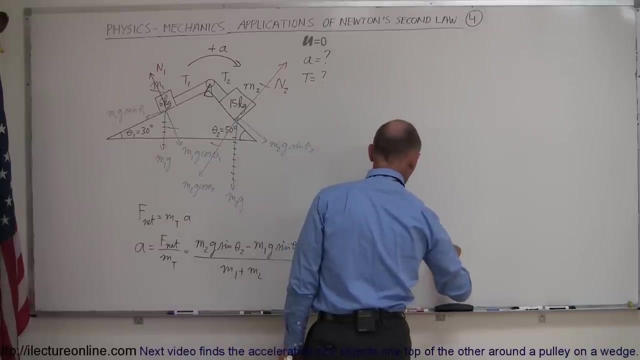 The total mass, which is m1 plus m2.. That would give me the acceleration of the system. Let's plug in the numbers. I'll leave out the units to make it a little cleaner. m2 was 15, g is 9.8, and we have the sine of 50 degrees minus m1, which is 6, g is 9.8 times the sine of 30 degrees, which of course is 1 half. all divided by the sum, m1 is 6.. 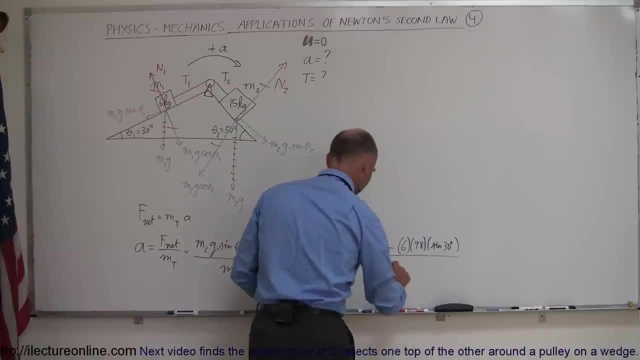 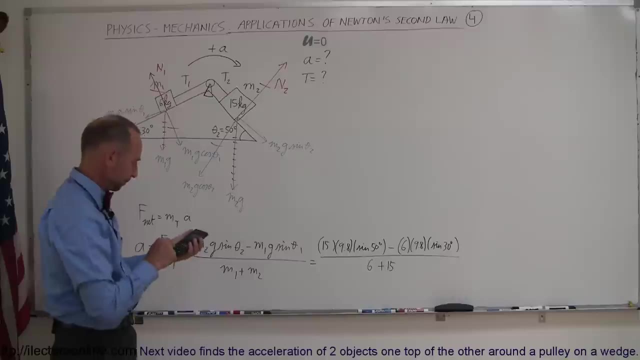 And m2 is 15 kilograms. So of course, then the units of this would be meters per second squared. So with a calculator, what do we get? 15 times 9.8 times the sine of 50 minus 6 times 9.8 times 0.5 equals. and take that divided by 21,, the acceleration would be 3.96 meters per second squared. 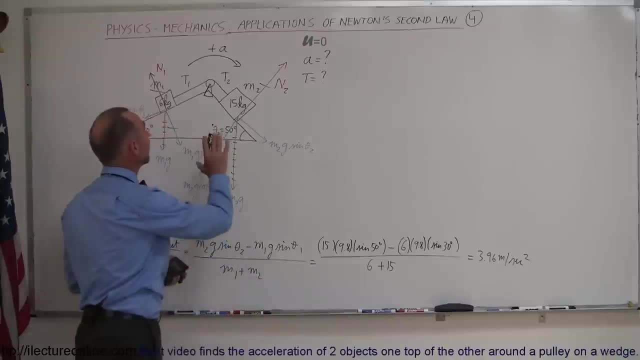 Alright, so now we found the acceleration. Now we need to find the tension in these strings. and of course we should already know that t1 equals t2, assuming that there's no friction in the pulley and we consume no mass in the pulley, so we don't have to worry about its moment of inertia. 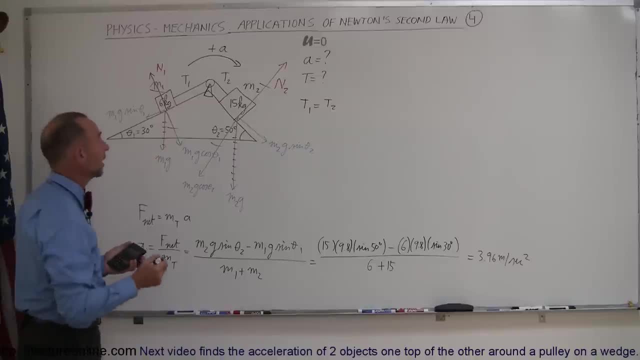 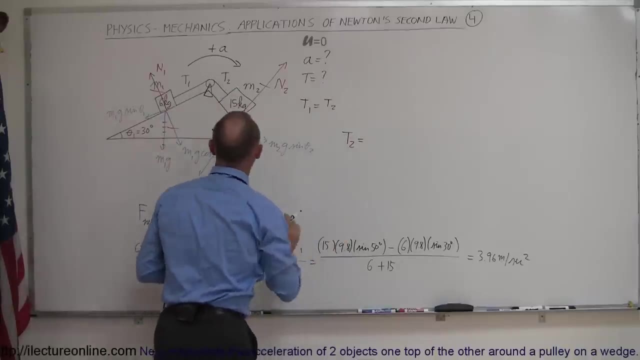 Alright. so what we can do now is we can simply say that the tension 2, I can do either way, but I'll start with tension 2,. tension 2 is equal to the weight component along the incline, which is m2 g sine theta. 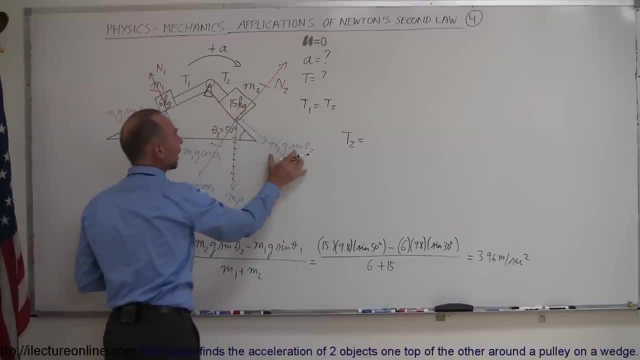 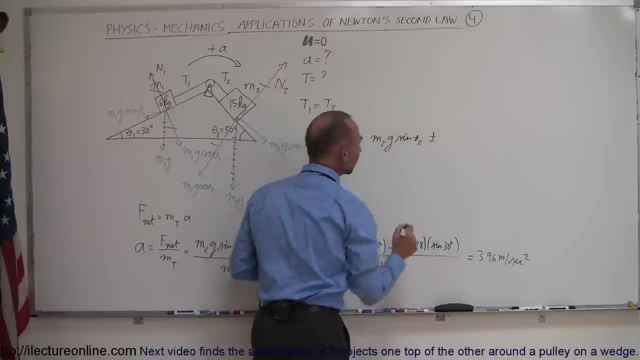 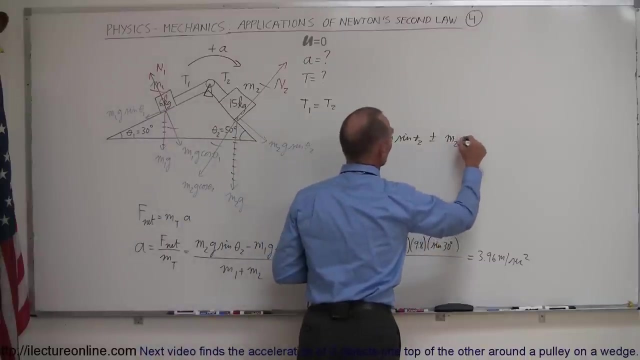 So it needs to have at least enough mass to hold up against its weight. So the m2 g sine of theta 2 plus or minus, and we'll decide if it's plus or minus the force required to accelerate this. So the force required to accelerate m2, with acceleration that we found the 3.96 meters per second squared. 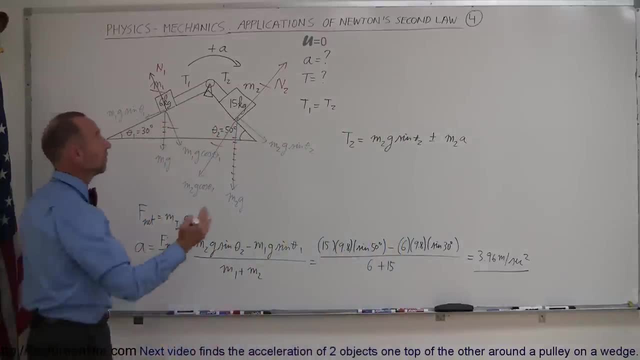 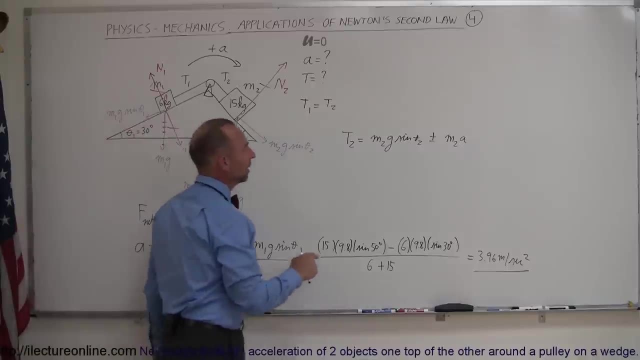 Now, is it plus or is it minus? It would be plus if the mass was being accelerated upward. It would be minus if the acceleration is allowed to go down. It would be minus if the acceleration is allowed to go downward with the force of gravity. so in this case we can say that it's going to be minus. 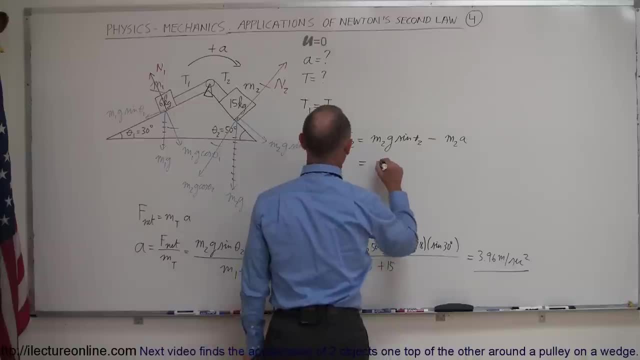 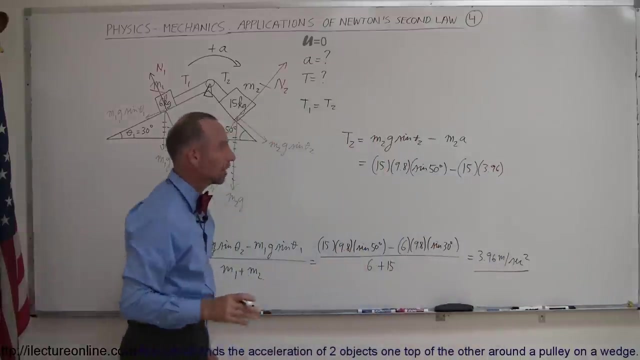 Now we plug in the numbers: m2 is 15, g is 9.8, sine of 50 degrees minus m2, which is 15 times acceleration of 3.96.. And again, units would be, of course, newtons, in this case.